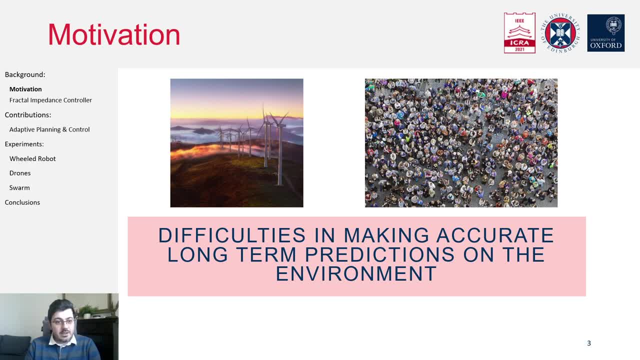 in the hope that we can reduce the cost associated with deploying our system into those scenarios, While still we envision to rely on numerical optimization to solve long term problems where, with the simplified models which are not computationally expensive and can be solved online in our system. 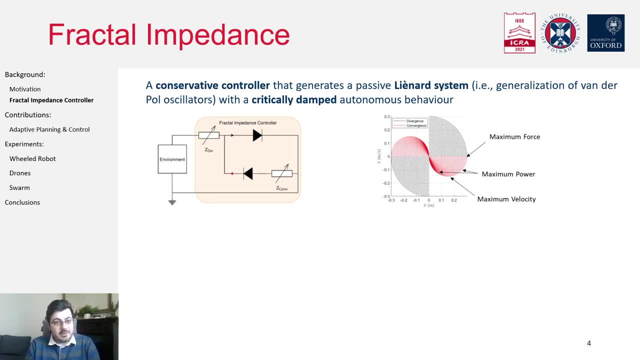 At the core of our solution. there are the fractal impedance controllers, which is a class of control agreement which is simple but rather complex, of controllers we have recently introduced. they use an algorithmic representation of an unarmed system to generate a critically dumped autonomous trajectory. a linear system is a system that is characterized by non-linear damping, and the most known are the: 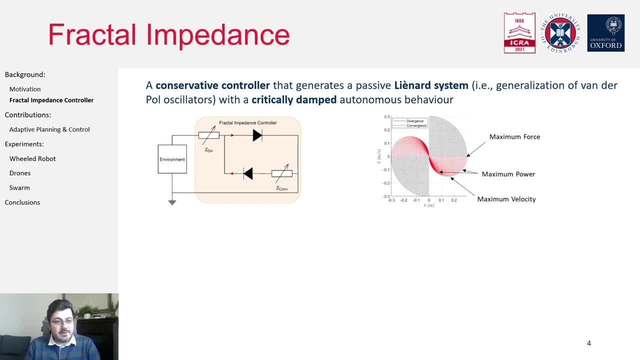 van der pole oscillators. in this case we don't have a direct formulation of the damping, but is generated by the logic present in our controller to generate the attractor, which is based on a diode, like elements which switch the lines through which flow the energy. 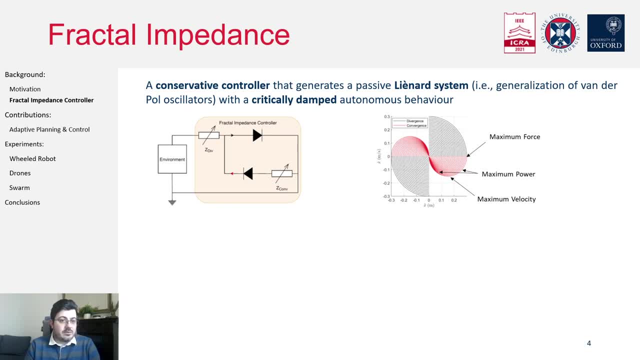 exchange with the environment during divergence and convergence, leading to an isotropic impedance in our system. so we can see in the schematic: when the system is absorbed energy by the environment, the only engaged impedance is this one and it will behave like any other impedance controller. however, when we the system starts to 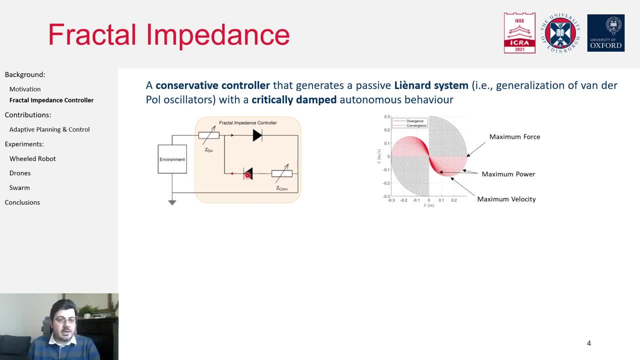 introduce energy in the environment because there is a reduction in the perturbation and it starts to converge to the search state, we will engage an additional impedance. the function of this additional impedance is to take this energy and redistribute the energy in order to obtain this critically dumped autonomous trajectory and go back to the desired. 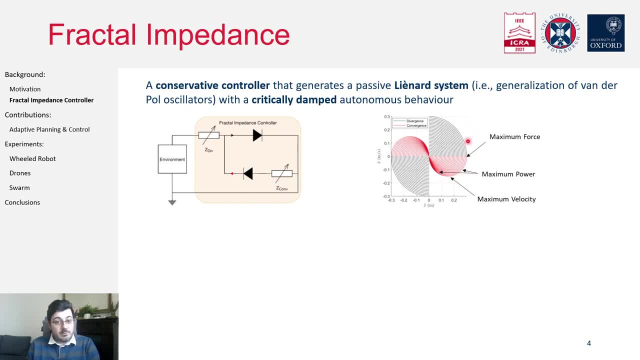 state. it's worth noting, these are trajectory harmonics, which implies that the maximum velocity is lower than a an equivalent minimum trajectory, which are the class of trajectory normally used in numerical optimizations, and I'm going to show you an example of how the trajectory is obtained and how it works. 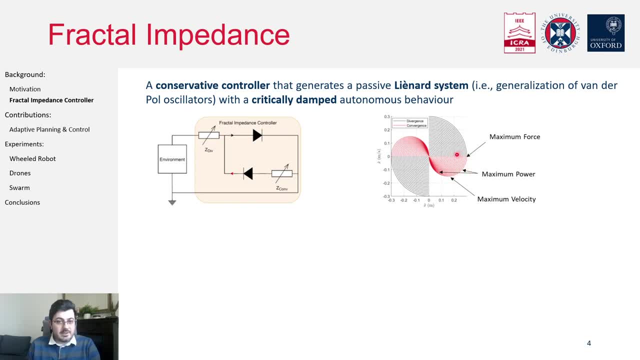 so the trajectory is obtained thanks to this algorithm: the maximum power that is released by our system and the maximum force. how does trajectory obtain? how this work? it's quite intuitive, and so we use the stiffness of our system as an observer of the energy exchange with the environment. 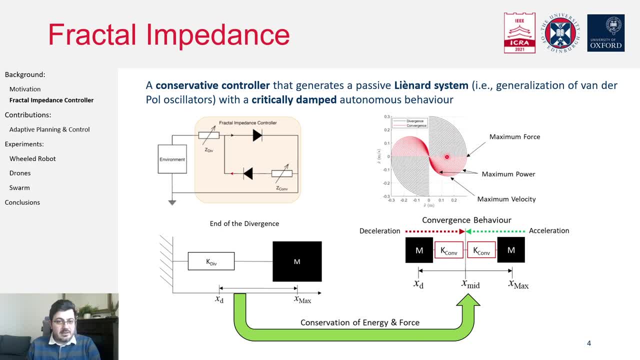 and then we apply the conservation of energy and force at the switching condition center in the midpoint, which will use half of the energy accumulated in our controller to accelerate the system and half of the energy to decelerate the system, reaching the desired state with the zero velocity. it's worth noticing that conservation of energy, conservation force can be. 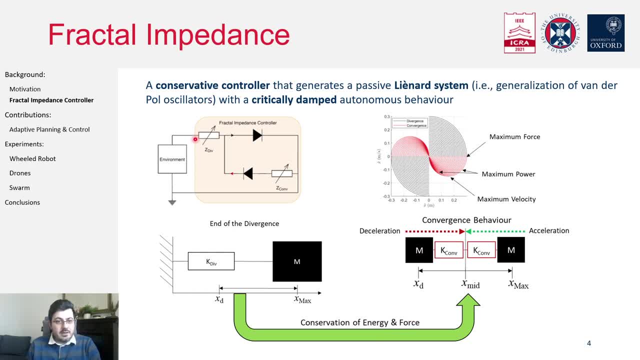 enforced at the same time only if the stiffness associated with the spring is constant. however, in case in case of a non-linear stiffness, then what we can do is introduce a virtual antagonist that will account for the jump in energy at the switching condition while enforcing the conservation of force, being this an algebraic solution to the problem? we don't have. 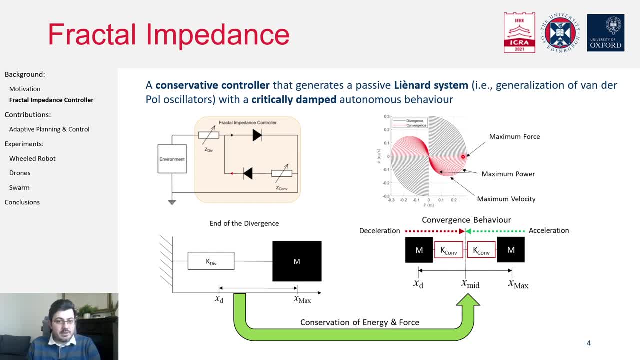 an issue with the stability, because it's a finite jump in the energy introduced into the environment and then consistent to obtain a system that is stable. furthermore, if we are able to bound those conditions to mechanical property of the system, we will obtain global regional attraction, which means that, regardless of the displacement between the desired state and the effective state, 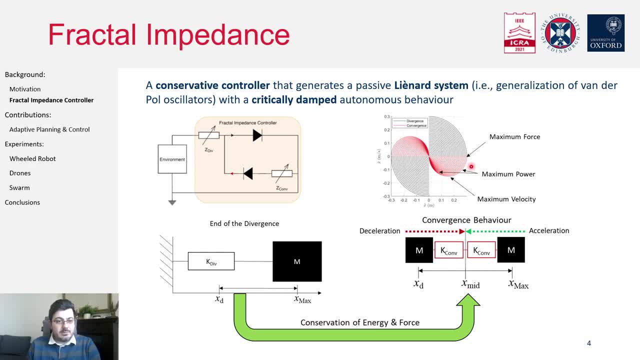 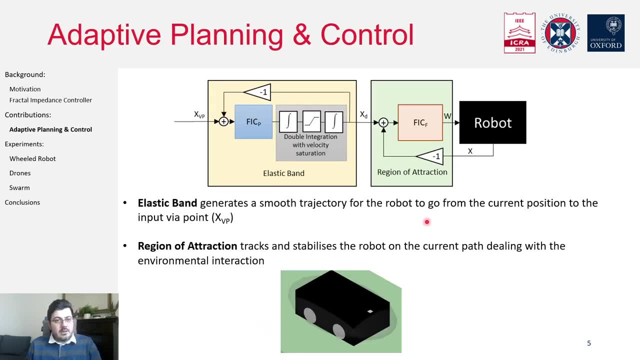 of the system- this is the controller- is able to generate smooth, autonomous trajectory to recover original state. then we employed this characteristic in our architecture, which is proposed in this paper, which have two of these controllers. the first controller is defined for unit of inertia, so we provide an acceleration in output which 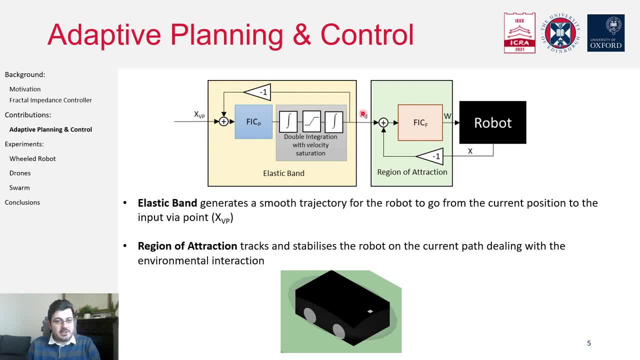 then is integrated two times to generate the desired trajectory, starting from an assigned via point, and then this desired trajectory is passed to a second controller which deals with the environmental interaction, both physical and virtual, thanks to an elastic bubble which is placed around the robot and generates a virtual potential field that can be used to avoid obstacles, which 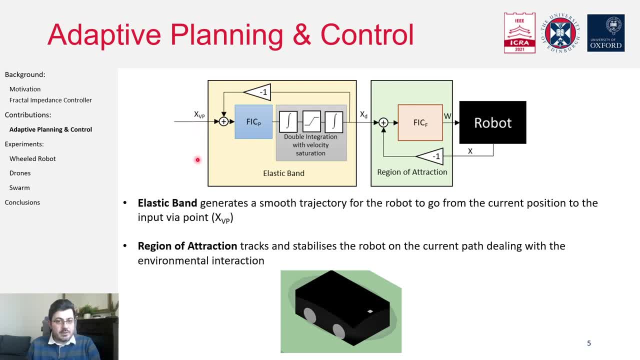 were not accounted in the issuing of the via points. furthermore, this could be also applied in velocity control robots, like in the real experiment we are presenting later on, by defining also this controller per unit of inertia, obtaining an acceleration command at this level and then integrating one time to obtain the. 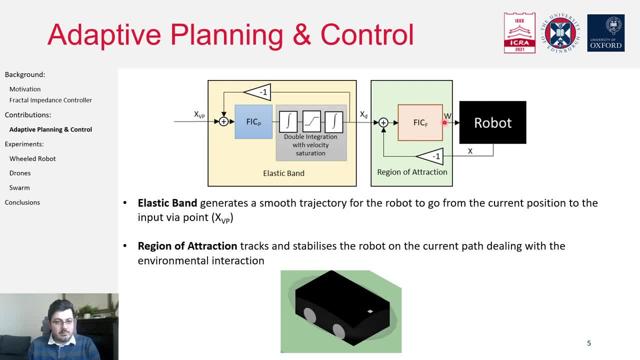 velocity command for the robot. however, it's worth considering that, doing this architecture in velocity control robot, it implies that in order to account for physical interaction with the world, we need the force torque sensor to measure the interaction. in contrast, if you're using torque control robots, we this. 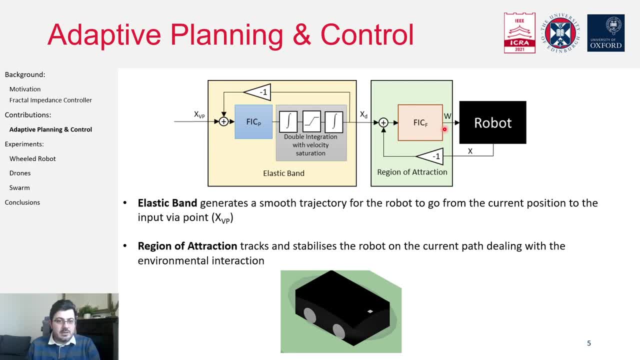 behaves like an impedance controller, and so it can autonomously deal with the interaction with the environment. in summary, we have an architecture which is composed by a cascade of two controllers: the first that generates the desired trajectory starting from an assigned via point, and then the region of attraction. 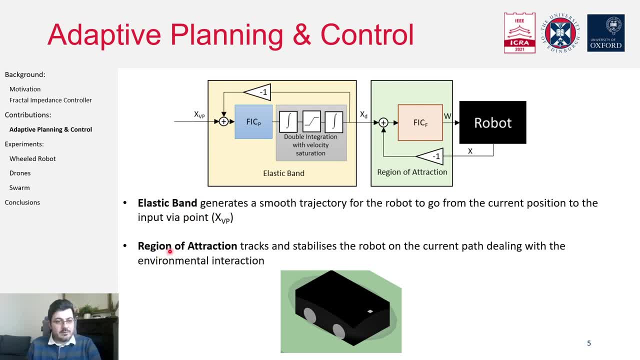 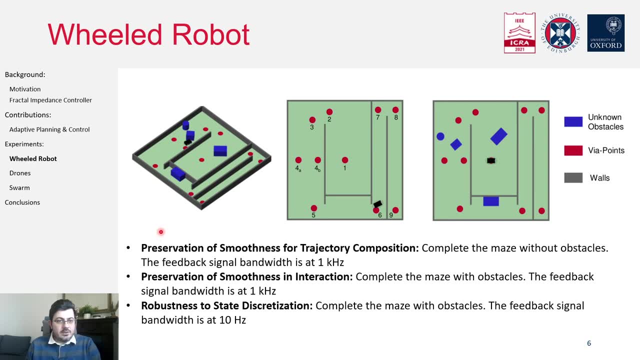 which is a second controller. we deal with the environment, interaction and tracking the trajectory. so the first experiment we are going to present is a maze. so we have an autonomic platform which is navigating a complex maze. so this is a non-convex domain which needs to be segmented in convex subdomains. 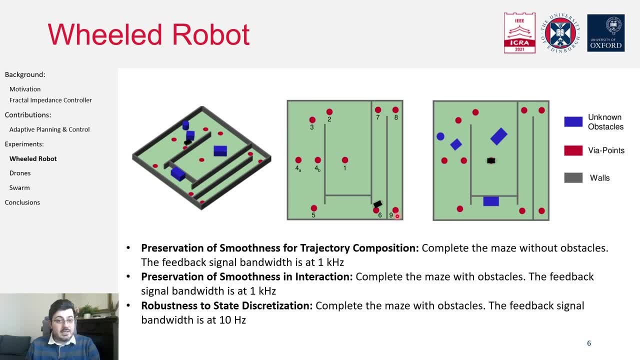 thanks to the assignment of via points. so in this case the via points are assigned manually, but they could be automated with multiple methods that are available to do geometrical segmentation in convex domains, and then we add some unknown obstacles in order to show that the region of attraction can deal with the present small concavity into the domain. 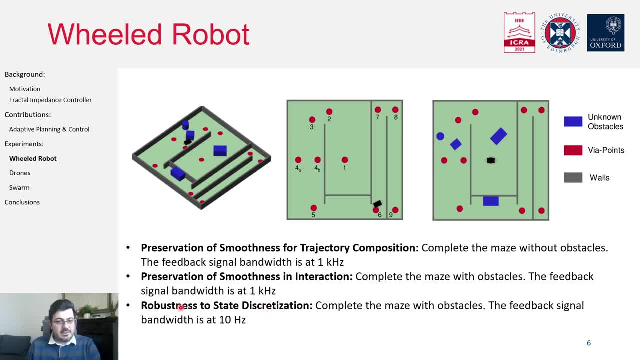 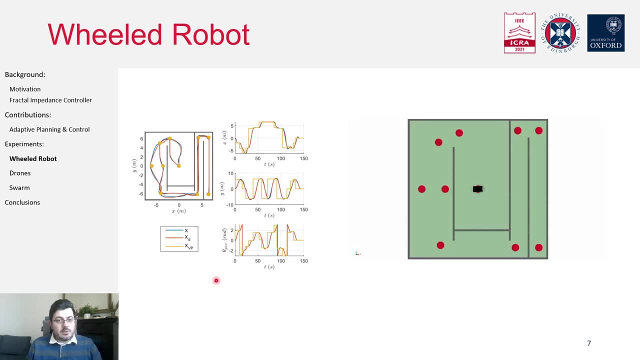 and lastly, the third scenario we tested is still with the obstacle, but we reduce the bandwidth of the feedback from the environment to 10 Hz and to see how this affects the performances in the region of attractions. so what we obtain in our results is that the system is capable of tracking accurately the desired trajectories. 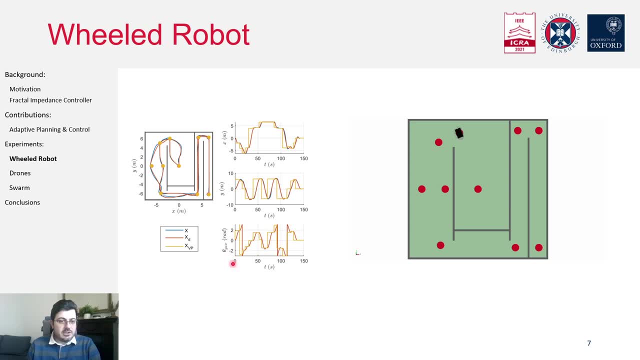 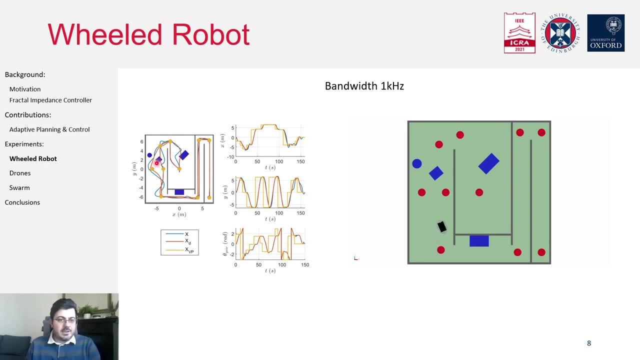 and the trajectory are smooth. these jumps here are not due to a non-smooth beam, but they are due to the wrapping of the angle into the rotation. when we introduce the unknown obstacles, we see that the region of attraction can adjust the behavior of the robot in order to navigate around those obstacles and complete the task. 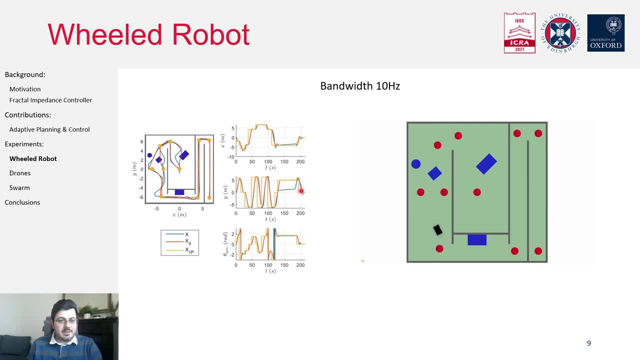 reducing the bandwidth of the feedback implies that the robot takes longer to go around the rotation the obstacles. however, is still able to complete the task. just that it will take a longer time to complete, but there is no problem on the smoothness or robustness of the trajectories. 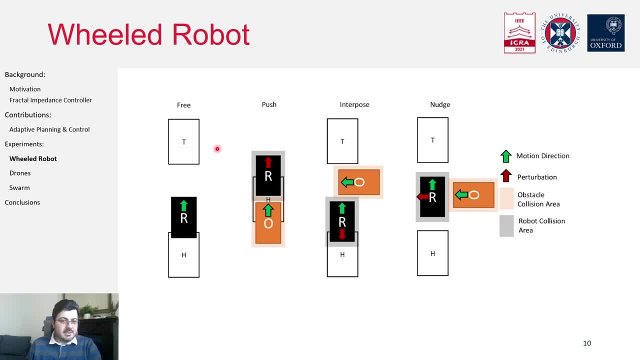 we tested this on a RIRAT system, which is a velocity control robot, as mentioned before, and we tracked the position of the robot in an obstacle using a Weigl motion capture system and the position of the two were measured. the virtual potential field pays around the two to generate a virtual interaction. 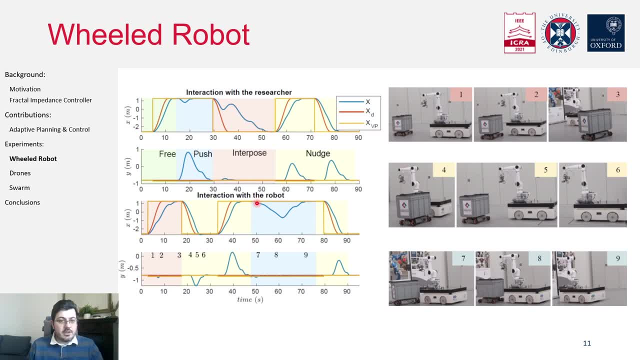 that, then, is passed to the region of attraction, and what we observe is that we are able to achieve smooth, autonomous behavior, both with the interaction with the researcher on top or with another robot below, and it's worth noticing how, in this case, we purposely set the elastic band. 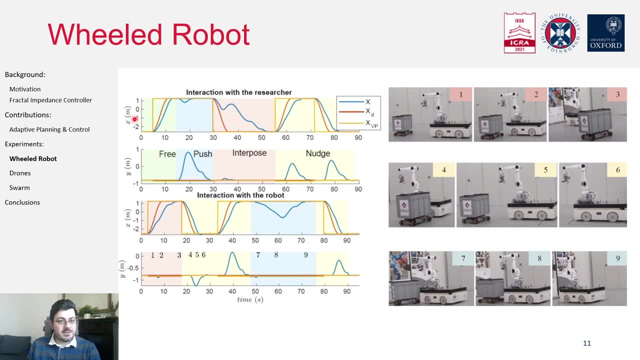 to exceed the mechanical property of the system, to show that if the region of attraction is properly calibrated on the mechanical properties of the system, then what will happen is that this system will still follow with the smooth trajectory. the desired path, however, will go at its own pace without affecting the system stability. 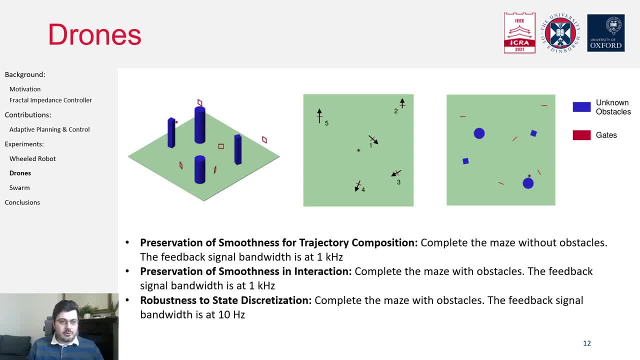 then we also test our architecture on drones which have six dimensions compared to the three-dimensional state of the mobile base, to test the first level of scalability of our controller. and we switch from a maze to a circuit with the five gates. each gates were assigned two via points to define the direction which the drone has to pass through the gate. 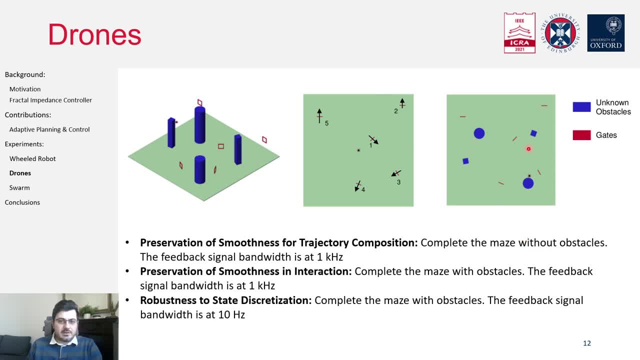 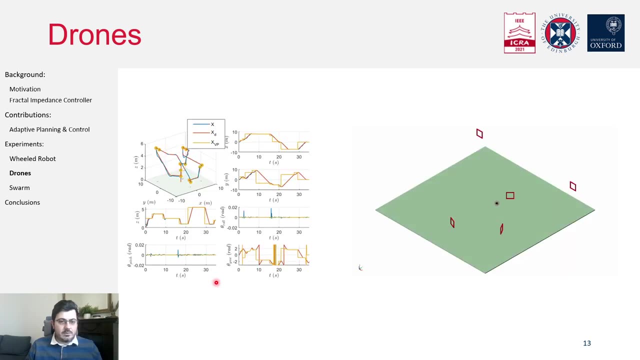 and then we added some maneuvers. we have known obstacles that the drone needed to avoid using the virtual physio interaction, thanks to the region of attraction. and then also in this case, we reduce the bandwidth of the feedback to 10 hertz. and what we observe? that still, the drone is able to navigate through the circuit without any problems. 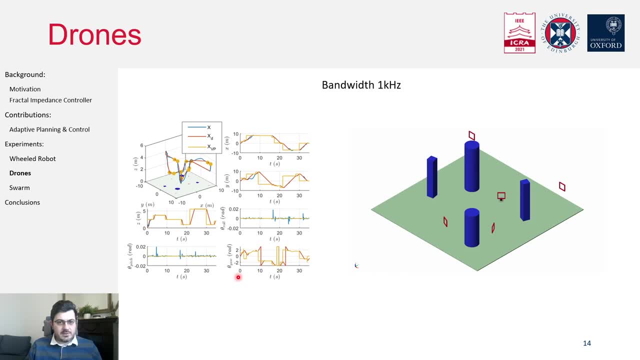 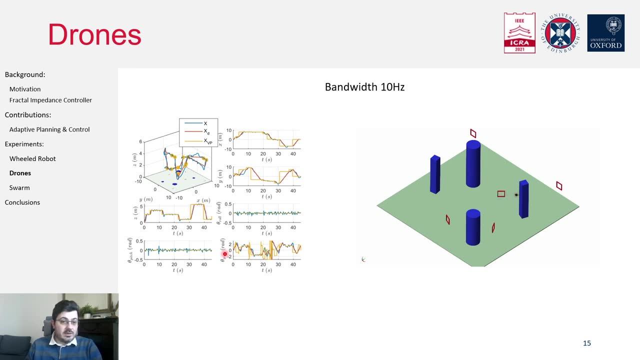 even in presence of unknown obstacles. however, when we reduce the bandwidth to 10 hertz, despite we don't have a problem with the drift of the system behavior. we still have smooth trajectories and robust interaction, but there is an higher fluctuation of the system states, comparable with an increased noise, due to the reduced bandwidth of the feedback. 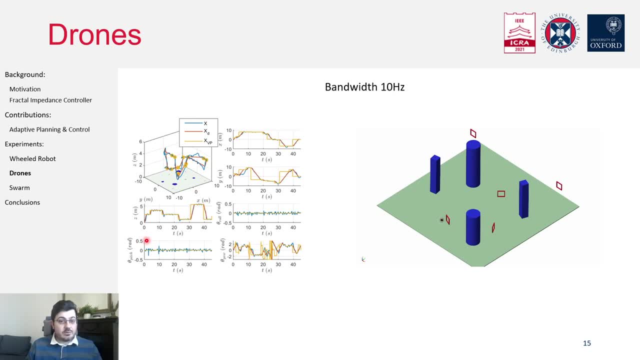 the fact that the controller is robust to reduce bandwidth but also to feedback delays, is due to the fact that we don't use velocity in our state, but the state is fully described by the position, which are immune to any problems associated with the observer state. in fact, the velocity are dependent by the observer velocity. 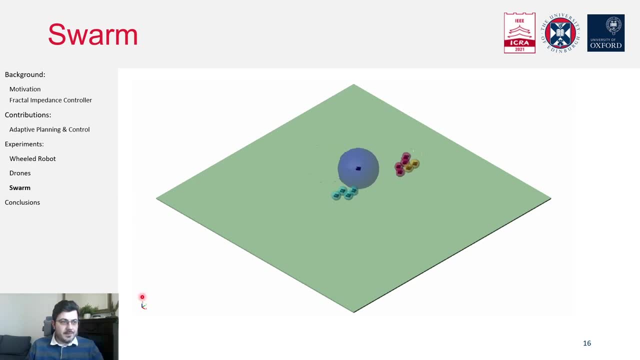 while the position are independent, are not affected by having a moving observer. then we also tested a sworn scenario where we had multiple drones synchronized by just assigning coordinated via points and while they were using this elastic bubble to interact and avoid collision among themselves while moving around, as well as escaping to the predator.